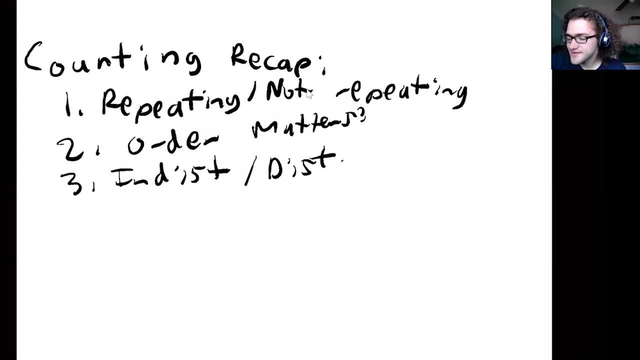 or distinguishable. So can I tell things apart, And so we'll deal with these latitude questions today. So we'll be counting things that have. we know that they're- they're not repeating, but we have to think about: can we order them or do we need to order them, and can we distinguish between these things? 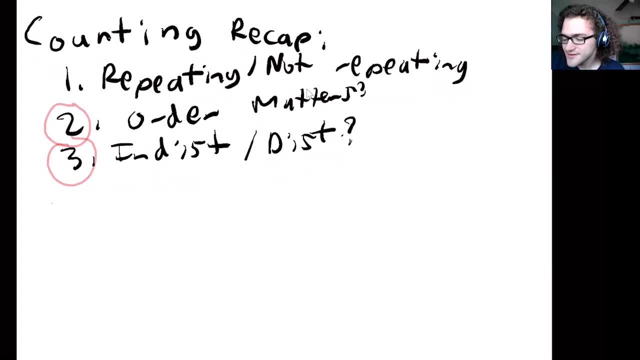 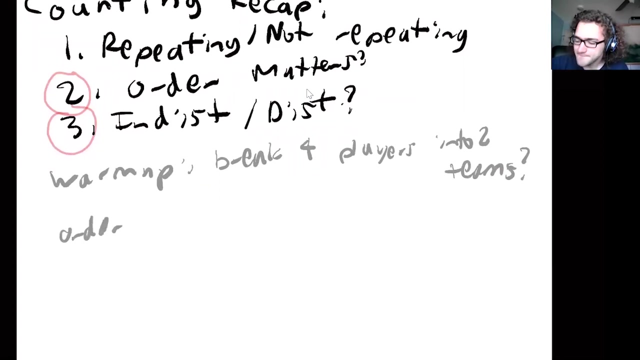 So as a little warm up, let's consider, we want to have, we'll break up four players into two teams, And so we want to say: how many ways can we do that? And so maybe initially we think, okay, well, does the order matter between players? 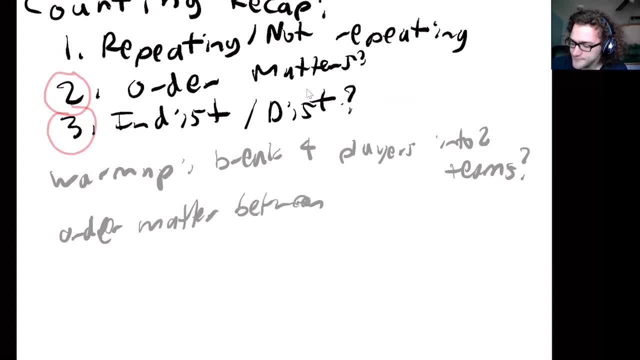 Like, say, if I had players A and B on one team and players C and D, Does that look different than if I had, say, B and A and D and C? Well, they're in the same team, so, no, the order doesn't matter. 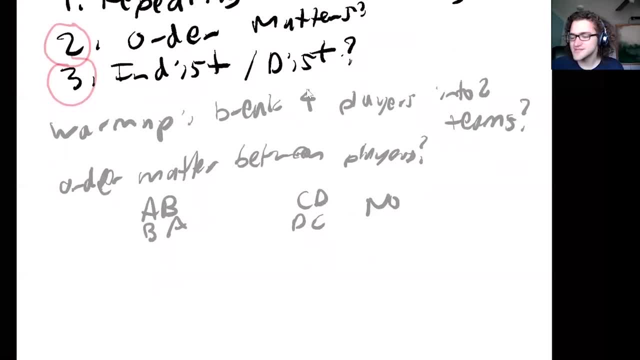 And so you might think, order doesn't matter, let's do combinations. And so maybe we say, okay, we have what we're trying to use with the order now, Which is смотреть what's too diyorsun. 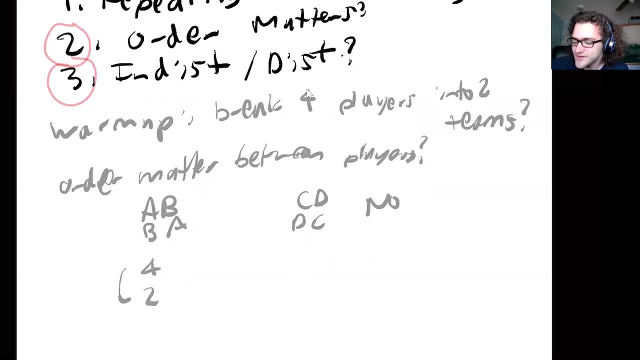 And we drive through. we're trying to parse, whether what we're- we're how we're sort of controlling or what we're creating- is reactive, where we're choosing out of four possible players and we'll choose two people for the first team and then we have two players left. 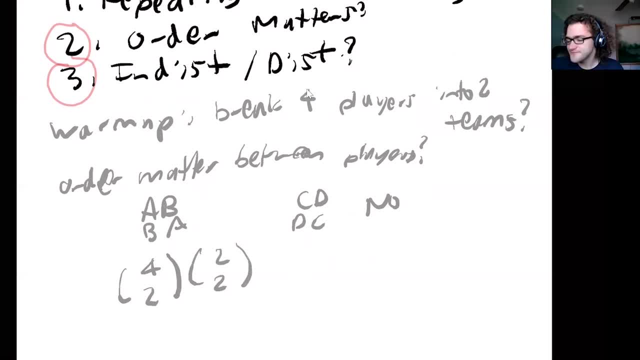 So we'll choose two players for the second team, In other words, like we'll have, and this two choose two is one. so we'll have just like four choose two, or four factorial, or two factorial, two factorial, or we'll have like six players. 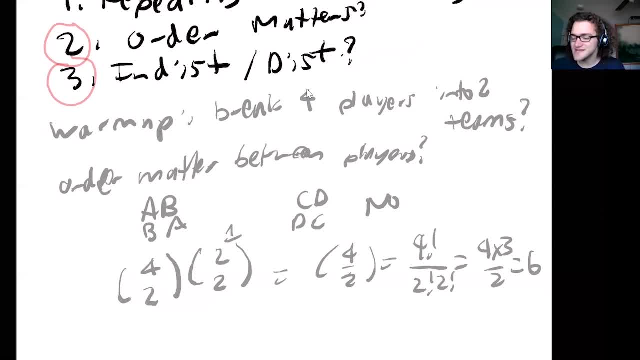 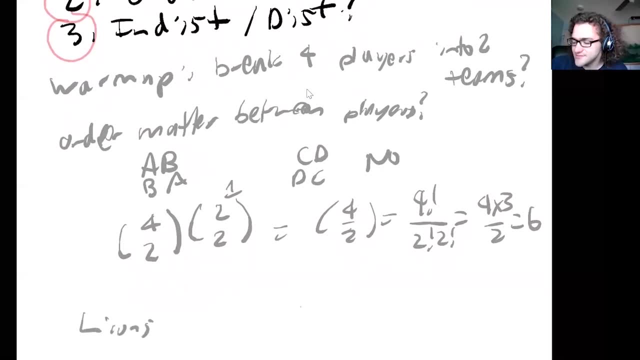 or six possibilities for this. However, we're kind of missing a subtlety here. So in this case I'm not really choosing. like I don't really have, say like a Lions team and a Tigers team, or I don't really have two teams that can distinguish. 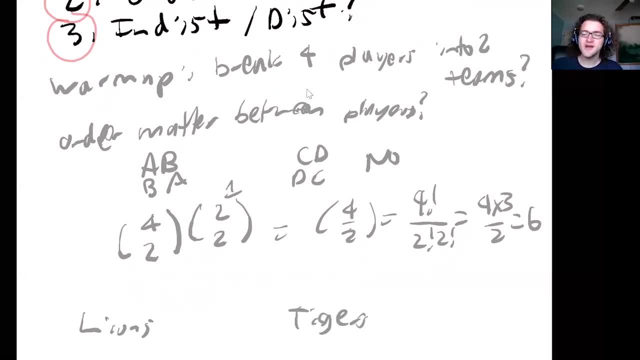 I'm saying, okay, the teams look the same to me. I'm just having one kind of team I don't know the name, another team I don't know the name for. So actually I have to divide by two to be able to not over count. 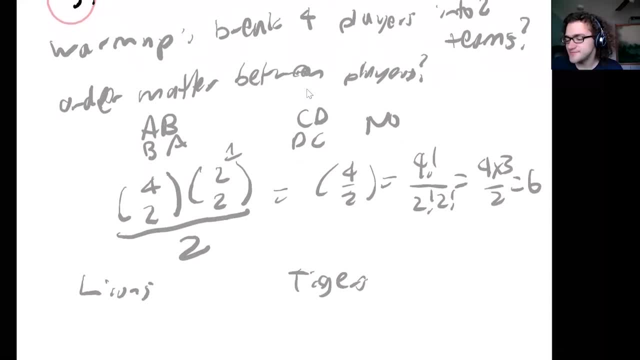 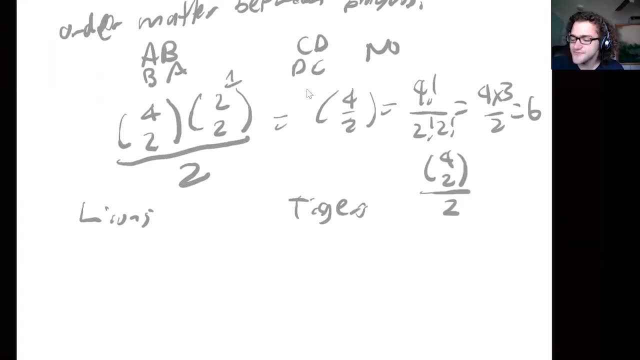 So here I don't care about the teams, And so it ends up being for choose two over two, Whereas if I'm saying okay, like let's choose players for the Lions versus the Tigers, Okay, here, then I have okay. 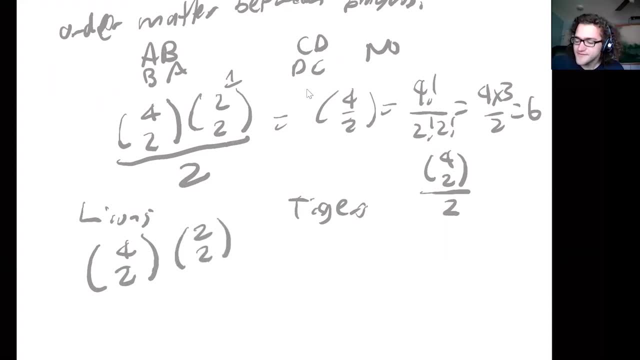 I can consider, okay, then I first choose players for the Lions and then I choose them for the Tigers, or like flip-flops, And so, yeah, that it becomes different if I'm having, say, A and B and the Lions and C and D and the Tigers, versus having 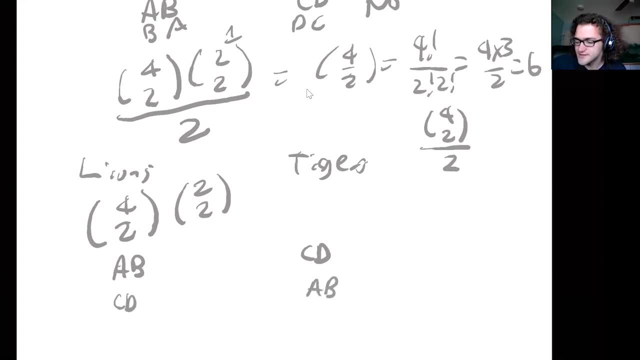 C and D and the Lions and A and B and the Tigers. it looks different, And so, yeah, so that's kind of one thing to be aware of here. So now let's kind of use this example and let's build on that. 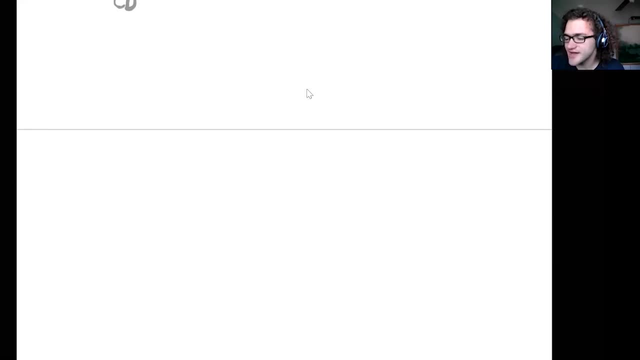 So we'll consider. we're wanting- you know, like you know, we have this time we have 17 players and we're wanting to say, okay, I'll have. we'll say we have, we have four teams and we know that we have like teams of. 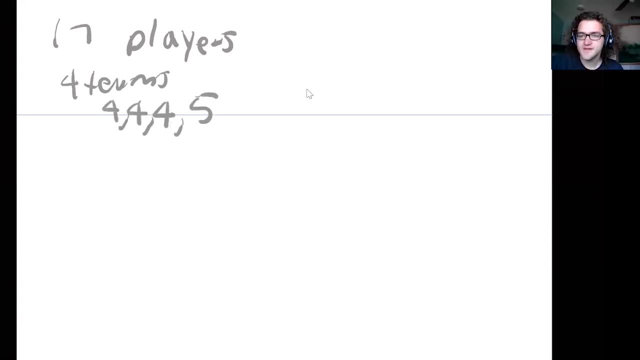 we have four, four, four and five. And so, yeah, thinking about this question, we might run into the same, the same situation where, okay, like if I can't tell the team apart, then say, like this team versus this team, a four. 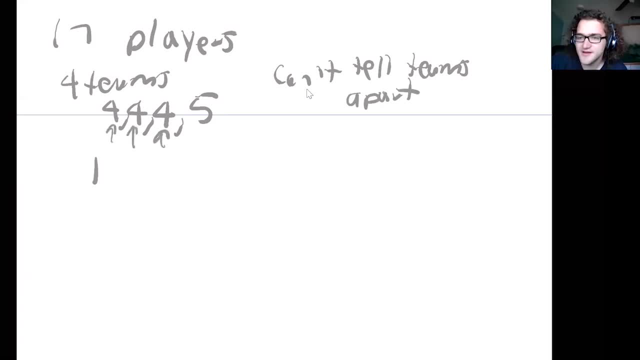 I can't, that doesn't matter to me, So I have to. I'll have to divide by all the number of ways I can order three teams And that's through How2ctorial I could. I could have kind of this idea of. 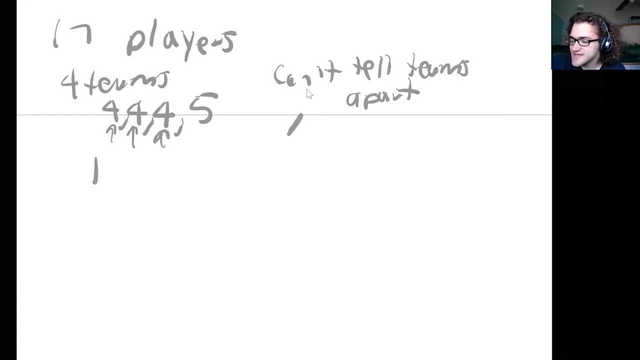 You know, I have this whole like do imaginar liquidez on the board, Like, yeah, I could bet altogether, Like I would bet 150 when I saw a receive and a drop Right. yeah, like i'm trying to order a few things. i have three factorial um, so i have to divide by that. 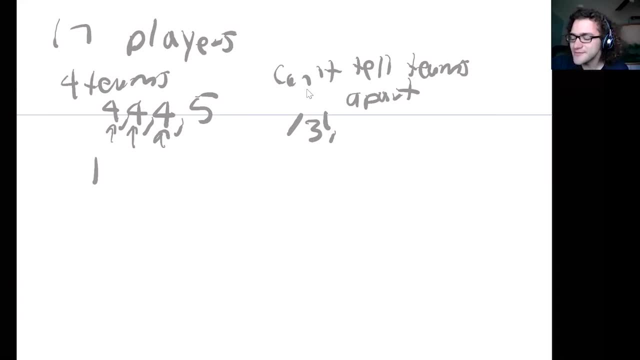 certainly, um, and now, how do i choose the players? um, a couple ways to do this. one way is: think about: okay, um, how long can you do it for? we start with 17 and i'll choose, uh, four players for, like, the first team, and then i have 13 left. then i'll choose four players, the next team i'm left with. 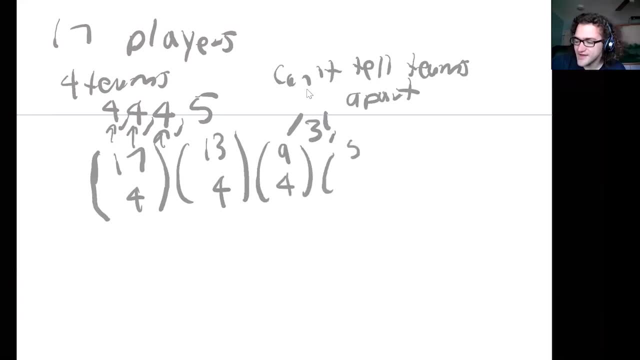 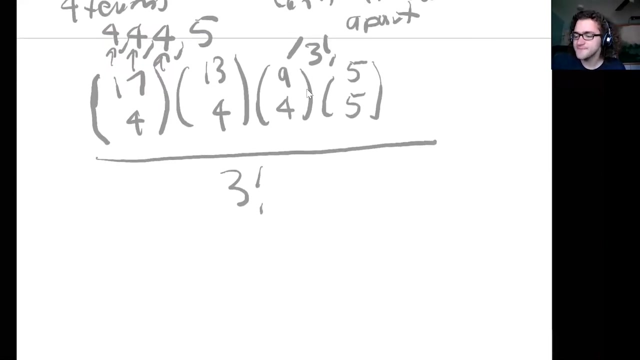 nine, then 13 minus four, so i'll choose four players and i have um, five players left, um, and i'll choose five for their remaining team, and then i'll divide all this by- uh, three factorial. i also can think about it as um, and this is an equivalent concept. so say, i have like 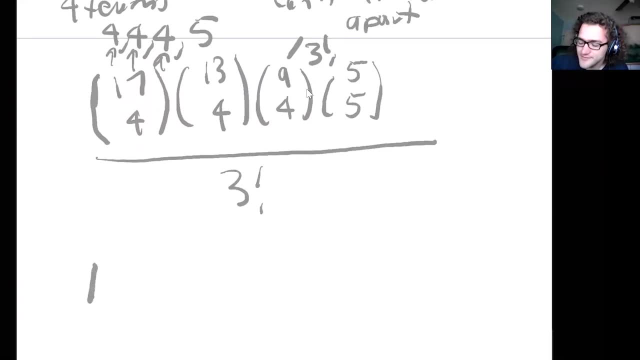 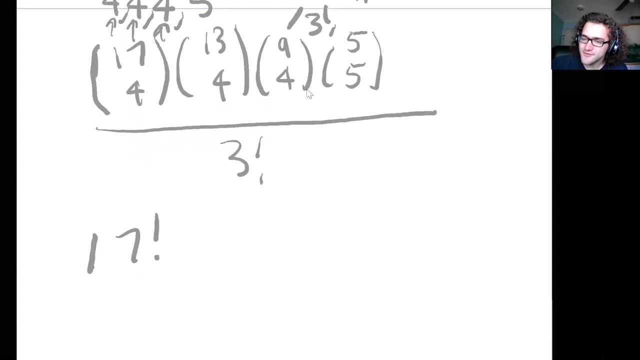 i'm gonna just like maybe order like all 17 players out in line and then um, i'll say, well, i have to consider, okay, what if i had? um. i'll do like divide off um by four, factorial right, because this is counting for, like that first team. 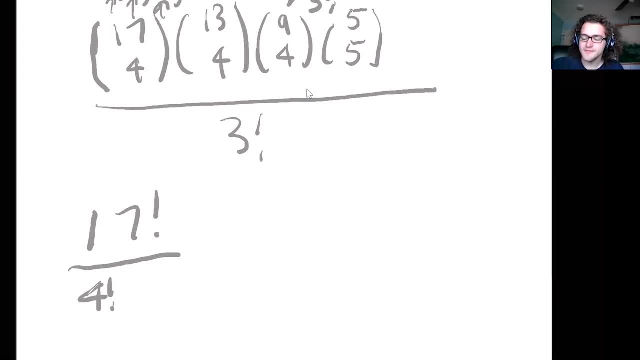 um, because i don't really care about the order among the players of that team, and then i have to divide out for the second team because i also have some repeating things. it's kind of like the idea of repeating letters, but it's in this case it's the players in the same team and then i do. 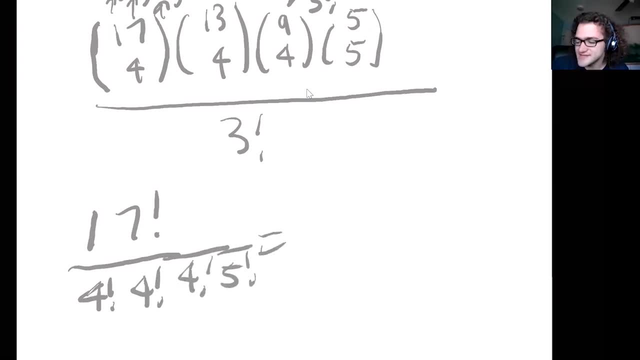 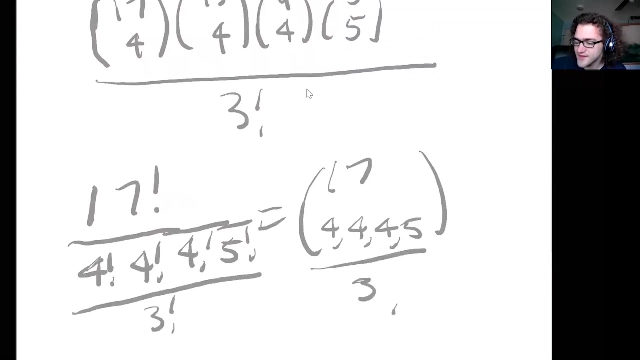 the same thing for the third, and then for the fourth, and then i can write this as um, the same indication as this, like multinomial coefficient of the 17 um, and then four, four, four, four, five, And I have to of course divide by three factorial here to make sure I count for the. 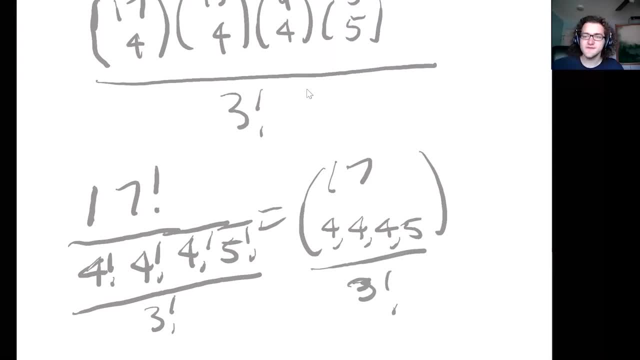 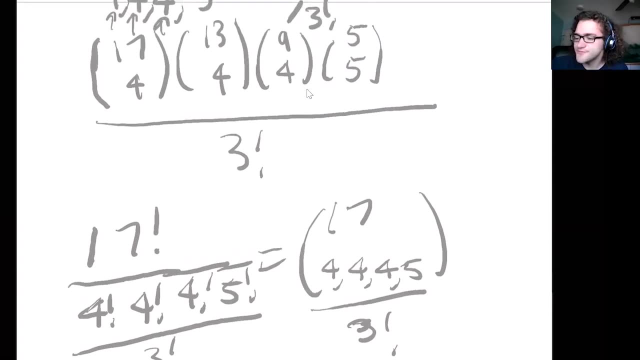 idea of, okay, the teams. I can't tell these, these teams of four apart, and there's three of them. So I have to order that, to not overcount, And so you can do the algebra to see: okay, if I multiply these things out, they end up being the same same number here and they're. 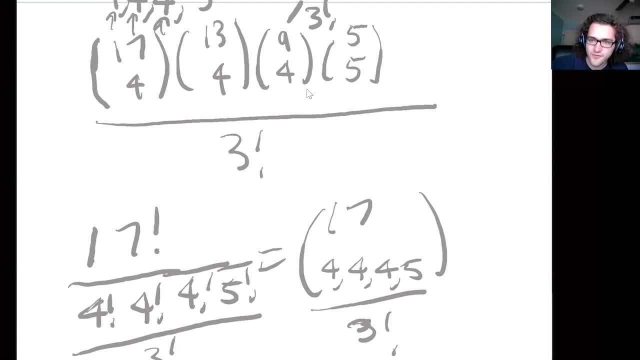 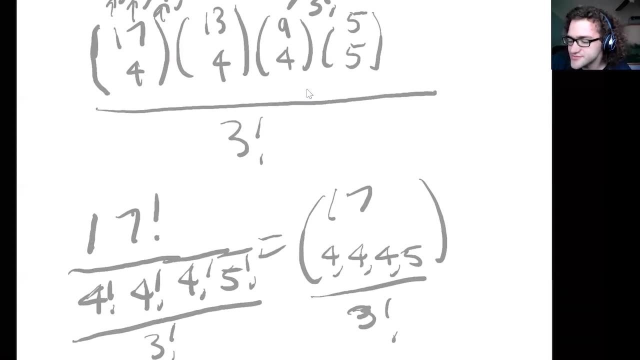 equivalent concepts of: okay, I'll have 17,, then I'll choose four, then I have 13,, I choose four as opposed to I kind of choose 17 all at once and then I will like choose these players more. 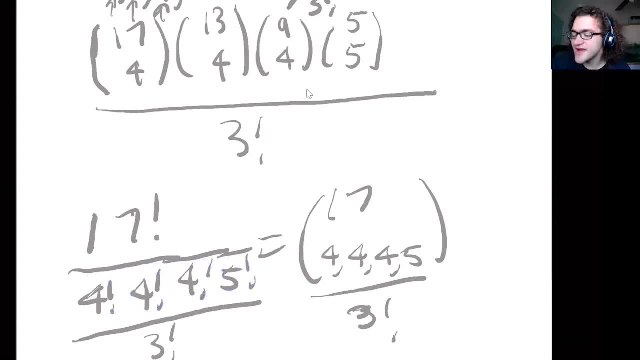 dividing them out individually. So let's say, what if? what if we actually did have teams? So let's say we- I don't know- take a hint from Wizard of Oz and we say, okay, we have like the. 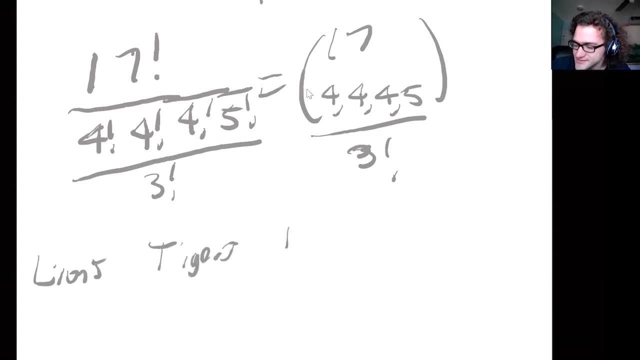 Lions, the Tigers, the Bears and the, the Oh My team, And so we can say: the Oh My has has five players, And, and so in this case, if we kind of didn't change anything else, we can still tell the. 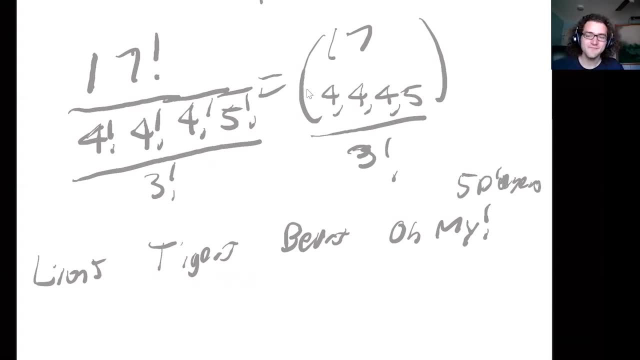 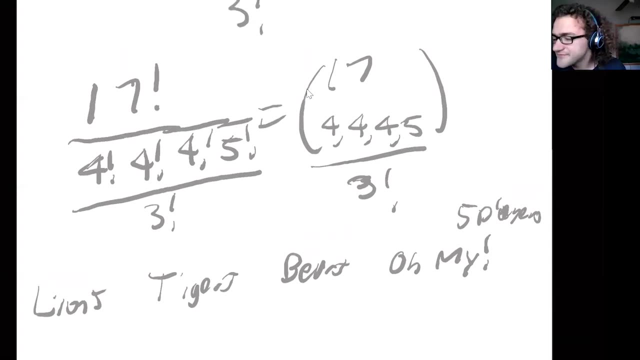 players apart, because, yeah, different people are, people are different, And so then we we end up with we either have like this idea of 17,, like the multinomial coefficient of four, four, four and five, or we can say, okay, 17,, choose four, 13,, choose four, nine, choose four, five. 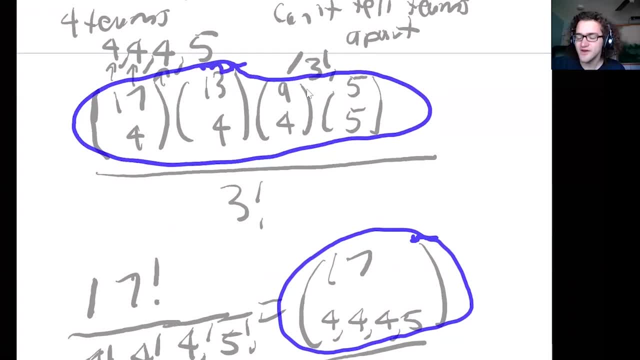 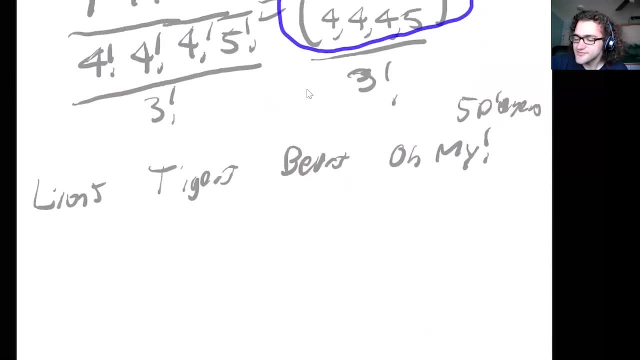 choose five. So I'm choosing, I'm choosing players for the teams and I can put them as between these teams of four apart because they're they're distinct. So that's how, how that problem would change if we could tell. 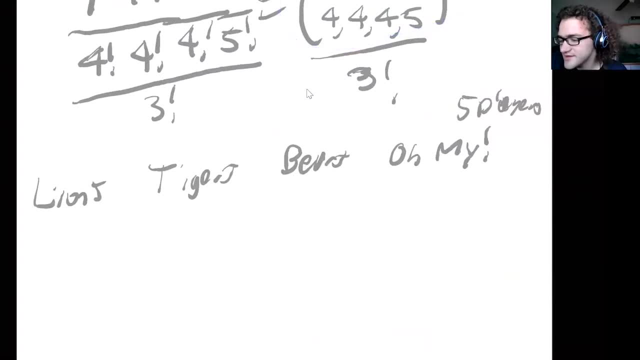 the teams apart. But let's consider what if we? we change the problem up in a more fundamental way. What if we say, okay, I can't tell the players apart, which doesn't really make sense. Let's, instead of saying players, we'll say: let's say we're, we're making these teams need to have. 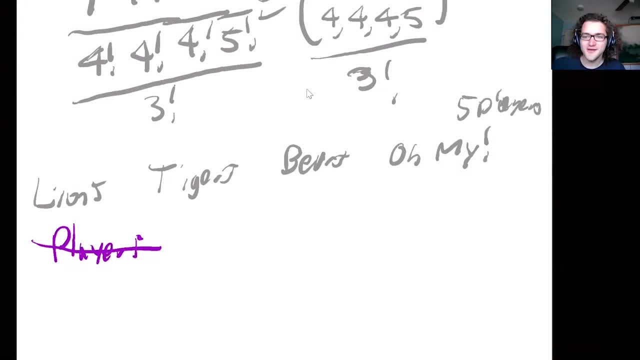 marching bands, right, And for marching bands, we need to have, we need to have, we need to have have drums. And so we're saying, yeah, we're giving, giving these teams drums, And so we can't really tell the difference between one drum and another drum. They look the same to us: Commodity. 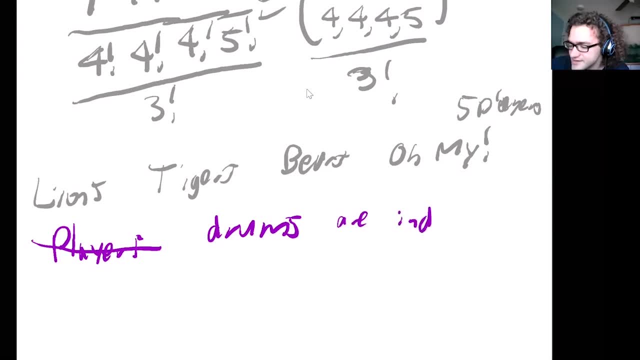 items. So drums are indistinguishable, But the teams are distinguishable. here I can tell the difference between the lions, the tigers, the bears and the. oh my, Okay, So then how does this change things? Okay, Well, this I kind of. at first this looks like: 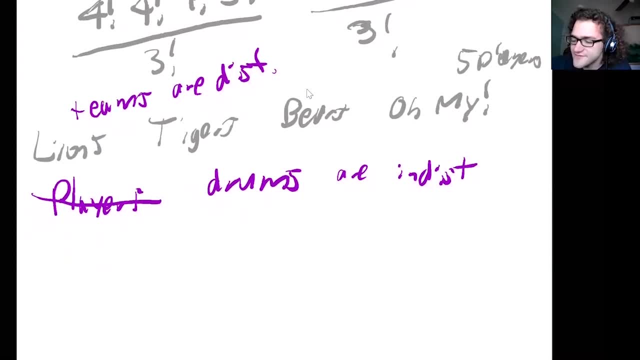 a stars and bars thing, right. It's like, okay, I have like these four teams- Those would kind of be, I can form my bars with them. right, It's like I have these start boards broken up by these bars. 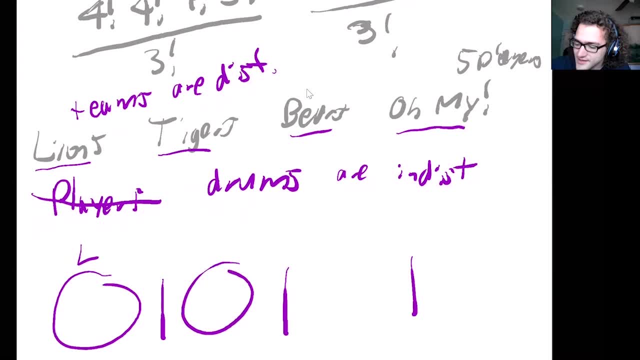 And okay, I say, here's like the lions board, the tigers board, the bears board and the oh my board, And so it's kind of like I'm just like I can think about it as I'm- I'm throwing the drums onto these dart boards And so, wherever it lands, 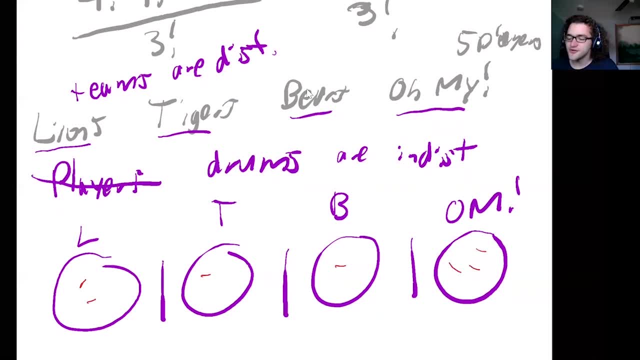 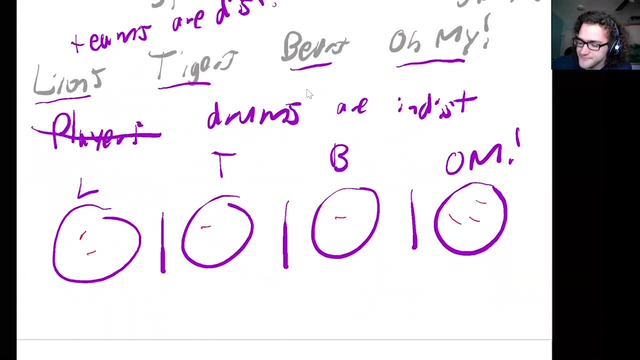 I like give the drums to the team And so yeah, then I can just kind of count up like number of stars, number of bars, And so I have, okay, I have 17 stars and I have three bars dividing these teams, So then I can say I have. 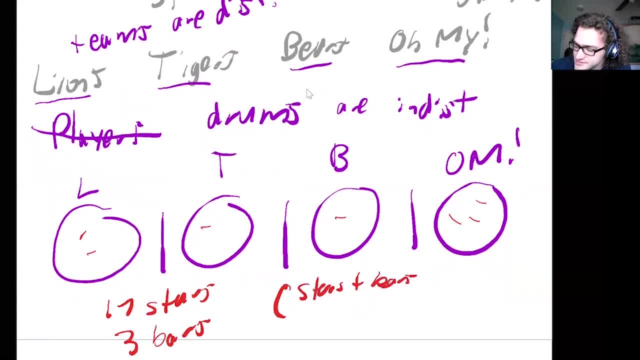 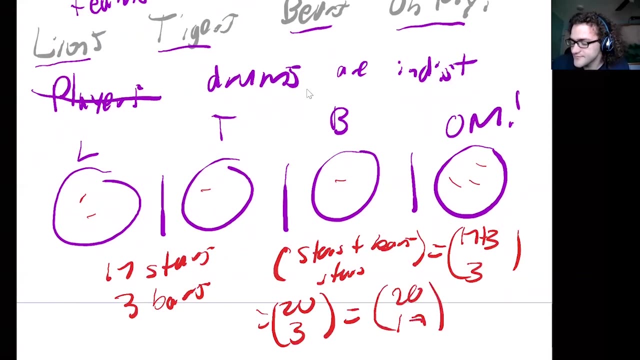 um, stars plus bars. Choose stars, and that's equal to 17 plus three. choose three, which is equal to 20, choose three, And that's the same thing as 22,, 17.. Okay, But that's. I've gone wrong somewhere right? Because? 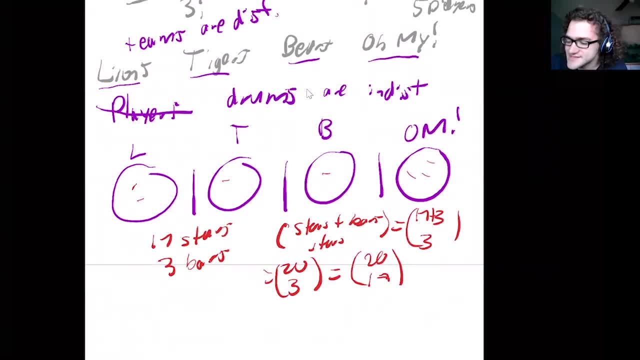 these teams. I've actually said: well, no, the lions here I'm allowing the lions to have anywhere from zero up to 17 people, But I have I said the lions have to be- you know, be- four. The tigers also are four, the bears are four and the- oh my- are five. 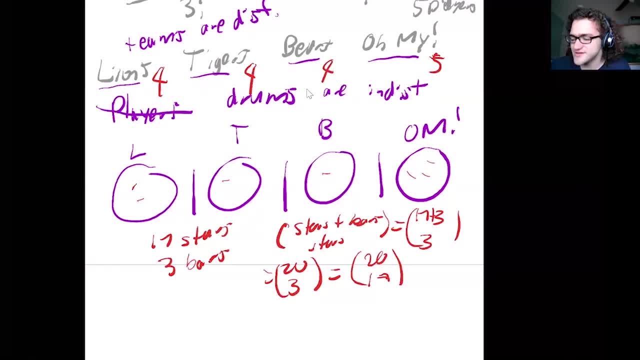 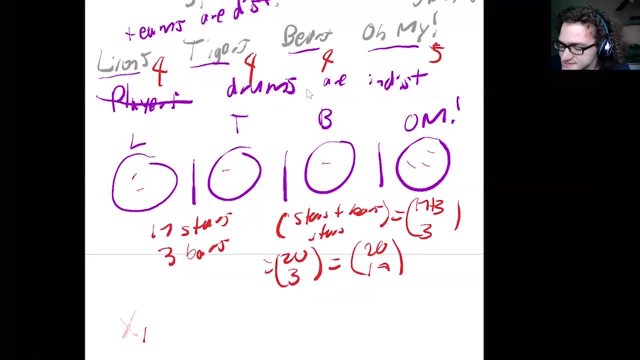 So, if you recall, like stars and bars, what is it solving? It's solving the answer to this question. We can say: okay, I have um, like some number of teams in the, in the first, and I'm going to be called that, And so the X, uh, we'll say, uh, team one, the players on team. 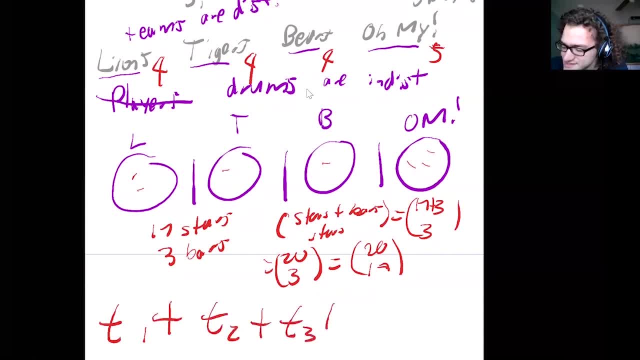 one plus the players on team two plus the players on team three plus the players on team four, And that's equal to 17 players, is what I'm I'm solving with this Um, this like 22,, 17 or 22,, three, um, with stars and bars, Cause I'm I'm kind of randomly throwing. 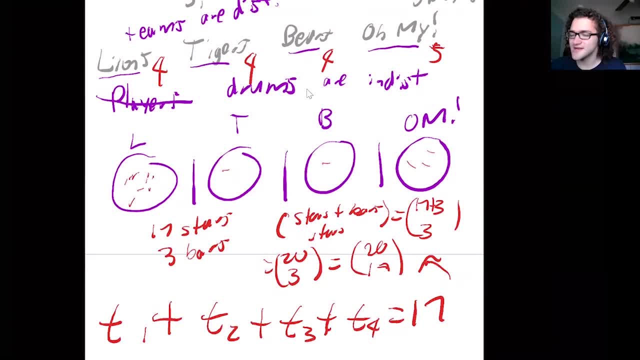 these drums um onto these like team dartboards, like I'm throwing yeah And there and then I'm kind of missing. okay, whatever it ends up like I'm, I have these stars and this bars, Um, but 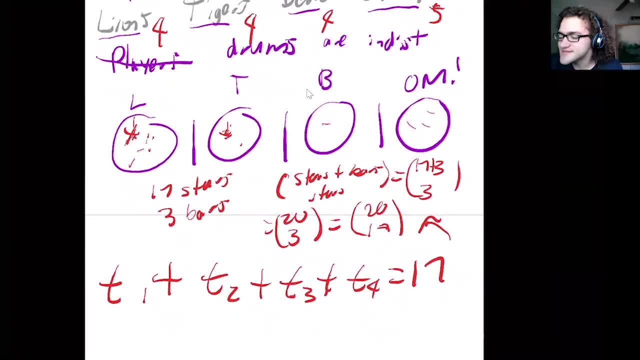 here um what I've done is: I've, I, basically, and I've said that I've, I know the team size, I'm not. I've actually already fixed my bar, my stars. I'm saying: okay, I know, I have. 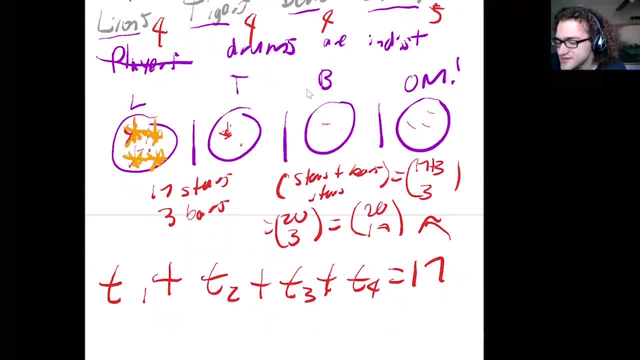 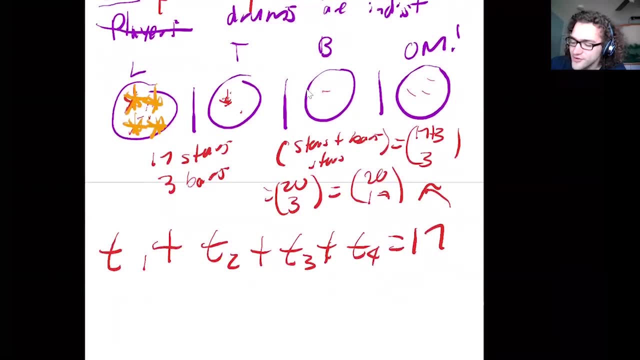 four stars for the lions. I know I have four stars for the tigers. I have um five stars for the oh, my team, And so, because I've already fixed that, I've said, okay, well, I know that, um, instead of having to count up all the possible teas, I know that.